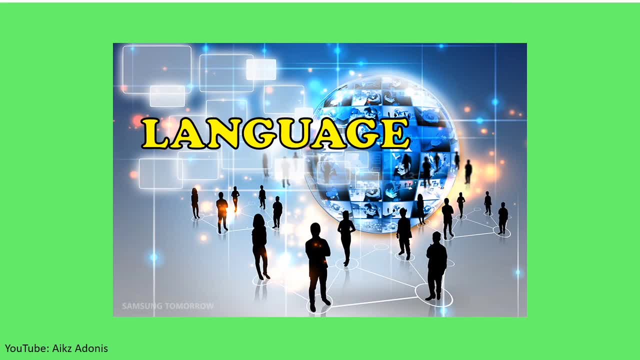 Mathematics has its own language which makes it easy to express its thought. Math is part of our everyday life. We use math in the grocery, in our work, school and even at home. In fact, we use decimal digit right after we woke up in the morning to determine the time. 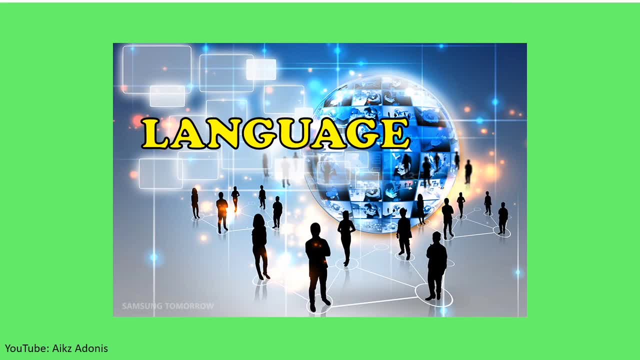 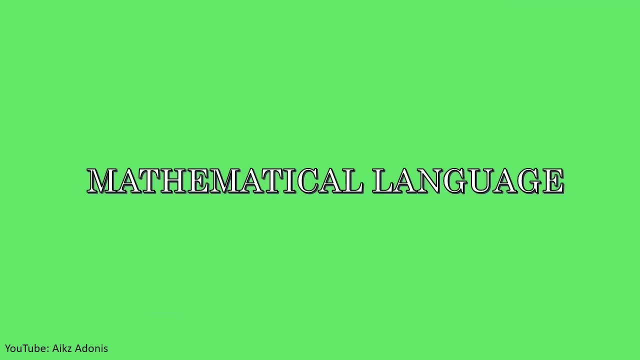 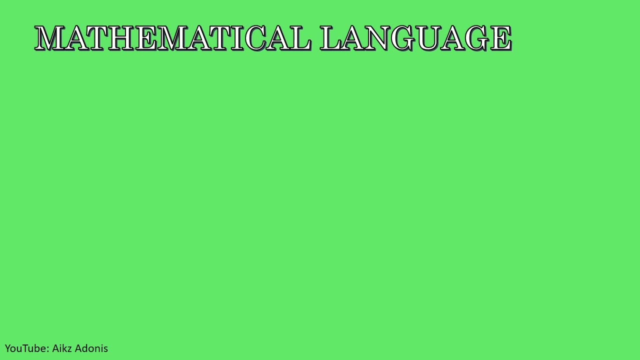 We really can't imagine life without math. Do you agree? I know you will? Why? Because even the number of years of your existence is an application of mathematical language. What is mathematical language or the language of math, by the way? 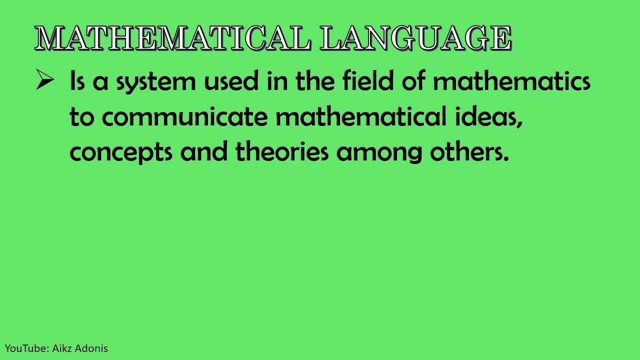 Mathematical language is a system used in the field of mathematics to communicate mathematical ideas, concepts and theories, among others. It is a distinct and unique form from the usual language that people are used to, And it is used to communicate abstract and logical ideas. 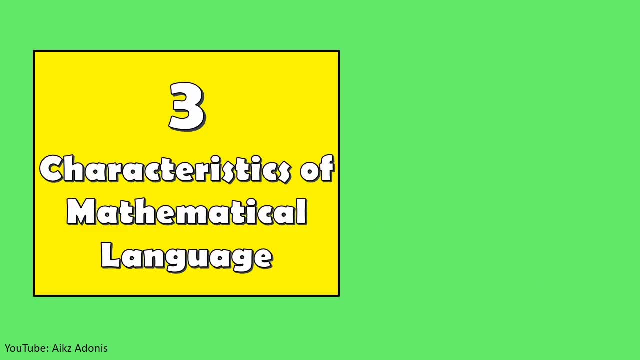 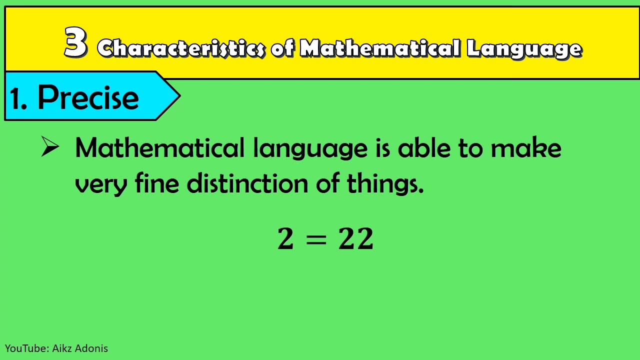 There are three characteristics of mathematical language. These are: being precise, concise and powerful. Mathematical language is precise. Precision of mathematical language means that language is able to make very fine distinction of things, And a little manipulation of symbols may mean a different thing. 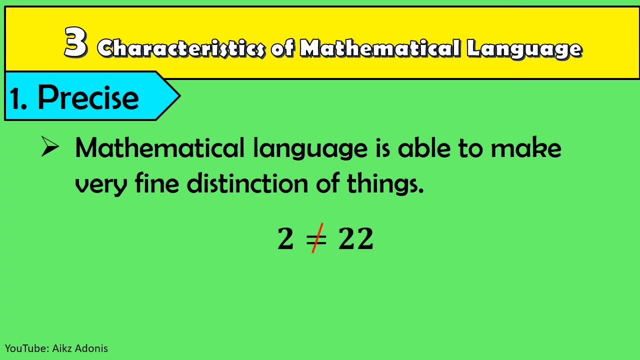 Like, if you will put a dash line across the equal sign of 2 equals 22,, it will mean a different thing. Mathematical language as being precise means accurate or exact. This is one of the reasons why math is considered as exact science. 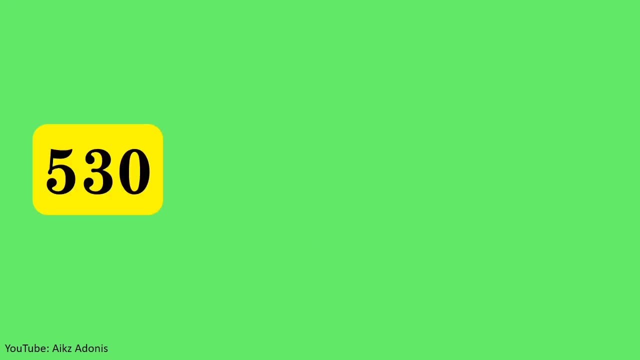 Numbers have many uses, so it is very important to know when and how to use them. For example, 530 will be read as 530 in the context of time, So it is very important to know when and how to use them. For example, 530 will be read as 530 in the context of time. 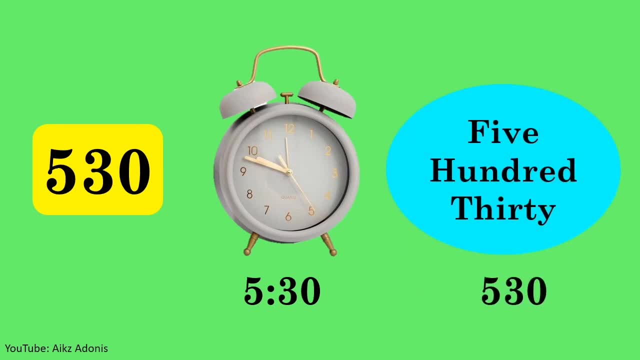 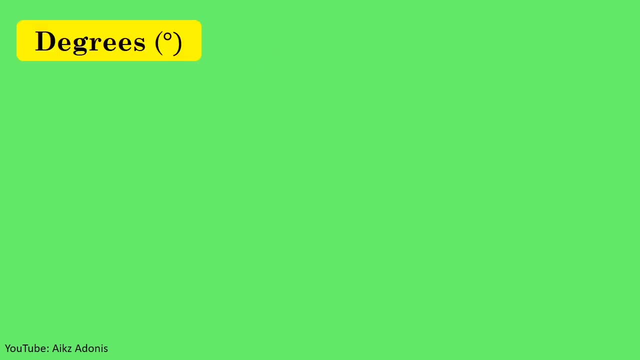 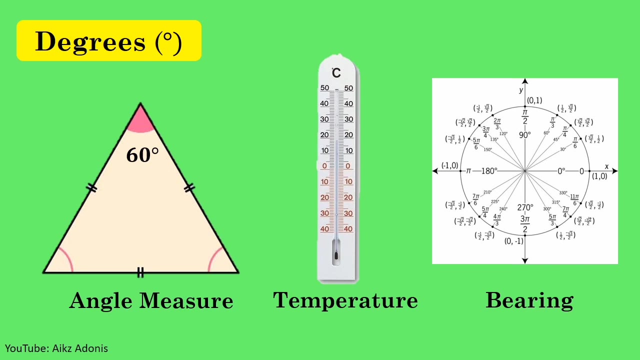 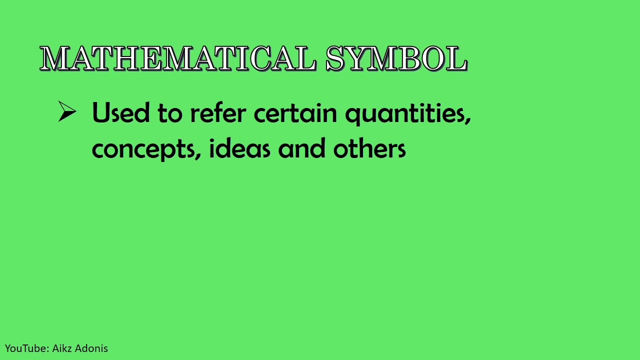 So it is very important to know when and how to use them. While 530 in the context of whole number, Another is different uses of degrees in angle measure in temperature and in bearing Degrees is commonly used symbol in math. Mathematical symbols are used to refer to certain quantities, concepts, ideas and others. 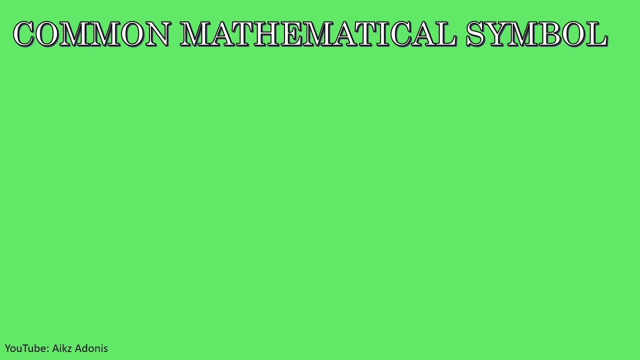 The most commonly used symbols in mathematics are degrees. The most commonly used symbols in mathematics are degrees. The most commonly used symbols in mathematics are the following: First, the 10 digits: 0,, 1,, 2,, 3,, 4,, 5,, 6,, 7,, 8, and 9.. 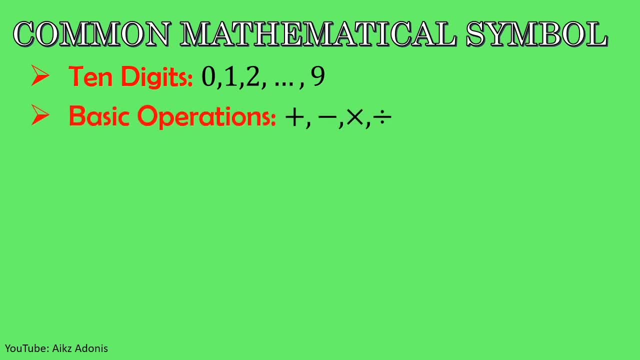 Next are the basic operations: Plus, minus, multiply and divide, And for sets we are using the symbols intersection, union, subsets and superset. Another commonly used symbols are variables. These can be any letter from the alphabet that represents a value or a number. 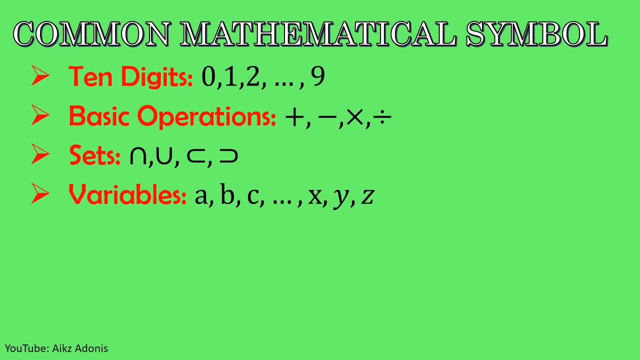 Usually small letters of x, y and z are used as variables. Special symbols like w for whole numbers, z for integers, q for rational numbers, r for real numbers and c for complex numbers. So these are the common symbols that we use in math. 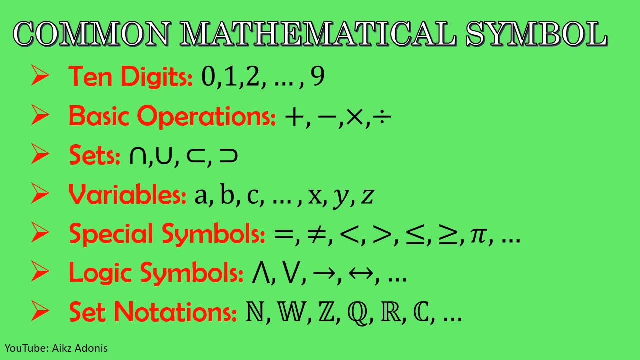 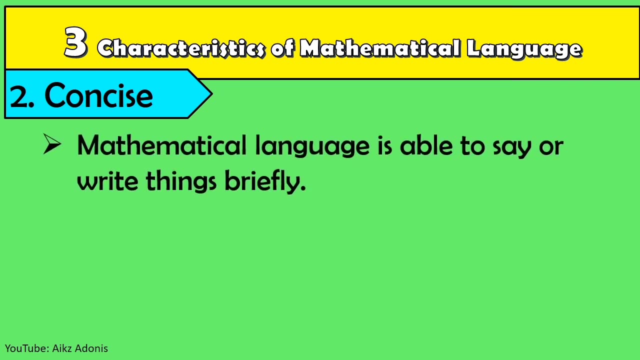 You must be familiar of these symbols so that it will be easy for you to understand the language of mathematics. Aside from mathematical language, as being precise, mathematical language is also concise, or being able to say or write things briefly. We can always convert mathematical language into equations or expressions. 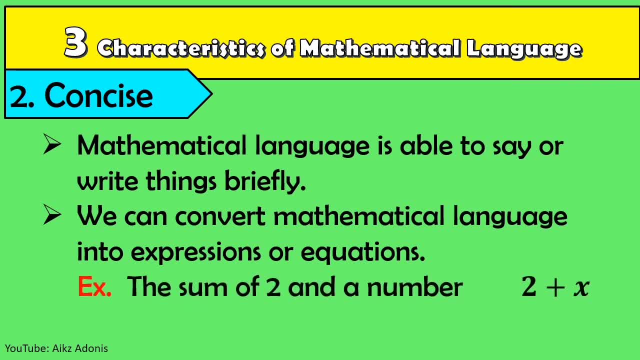 For instance, instead of writing the sum of 2 and the number, we can write the expression 2 plus x, wherein a number that is unknown is represented by the variable x. Another, instead of writing 5 times a number, we can write: 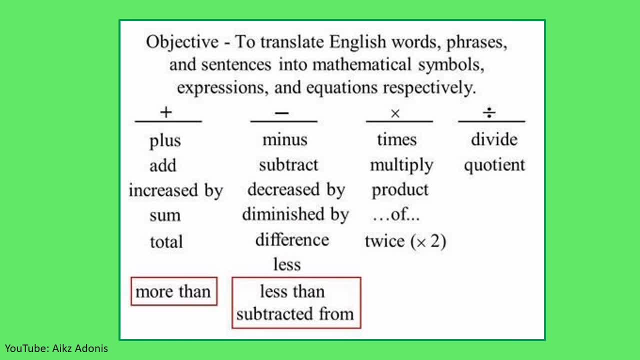 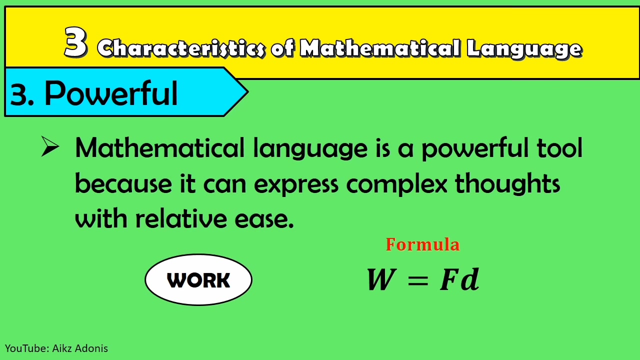 And here are some of the other English translation of mathematical expressions and sentences. Being familiar of these translations will help you in understanding mathematical language. Aside from being precise and concise, mathematical language is powerful. Mathematical language is a powerful tool because it can express complex thoughts with relative ease. 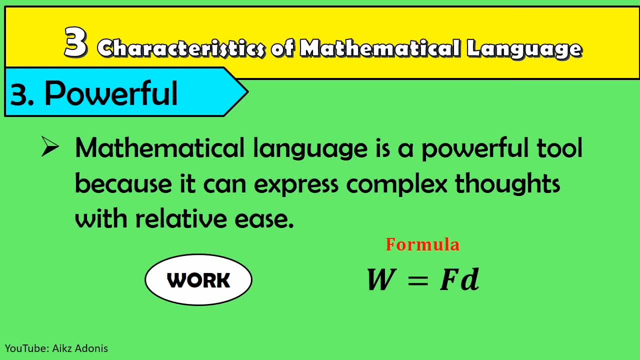 Using equations and formulas, For instance, work is an activity that involves mental and physical effort done in order to achieve a purpose or intended result. Now, what if we want to measure work so that it can be useful for different industries? This is possible when we use the formula: work is equal to force times, distance. 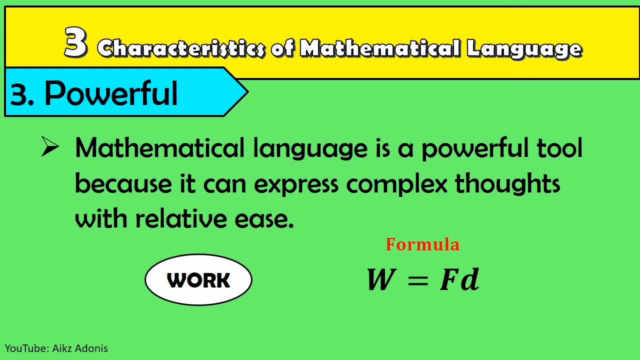 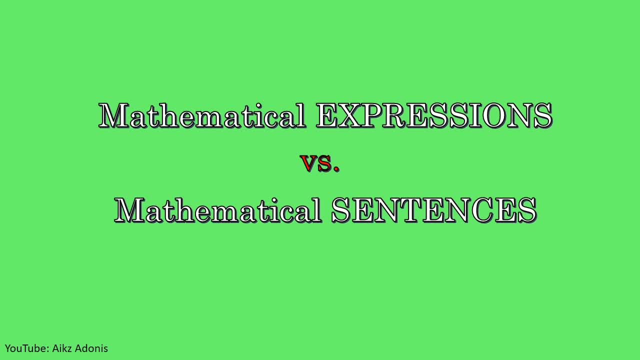 In fact, there are lots of equations and formulas which are used by mathematicians in discovering the world. Now let's talk about mathematical expressions and sentences. The combination of variables, operations, notations and symbols form a mathematical expression or sentence. 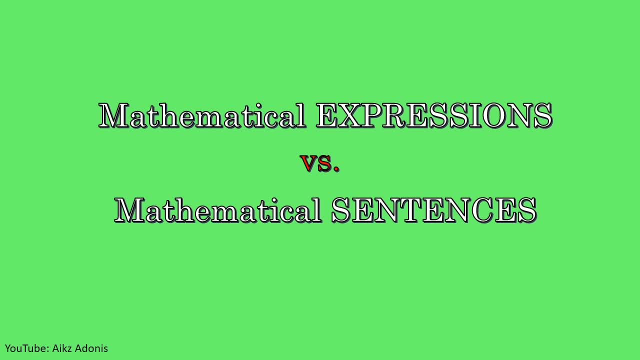 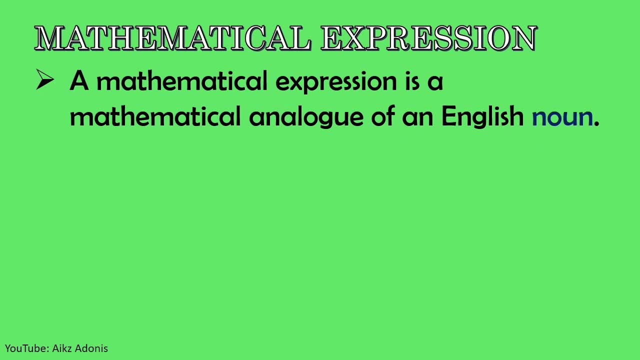 Now let's look at the difference between the two. A mathematical expression is the mathematical analog of an English word. A mathematical expression is the mathematical analog of an English word. A mathematical sentence is the mathematical analog of an English noun. It doesn't state a complete thought, and the most common expression are numbers. 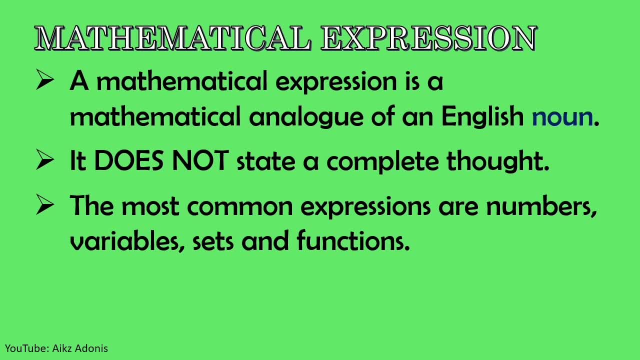 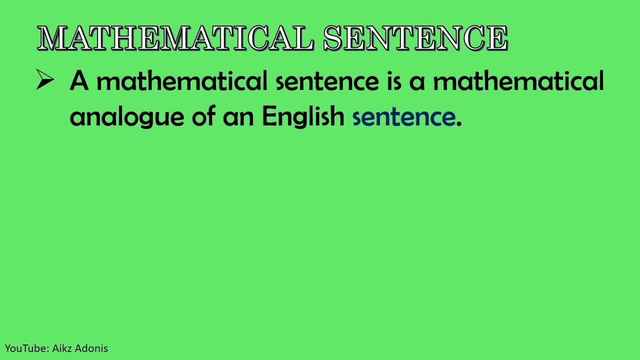 variables and functions. For example, five, 8x and y-3 are mathematical expressions. A mathematical sentence is a mathematical analog of an English sentence. It state a complete thought. For example, 1 plus 6 is equal to 7,, 8x is equal to 16, and x minus 3 is greater than 2 are mathematical sentences. 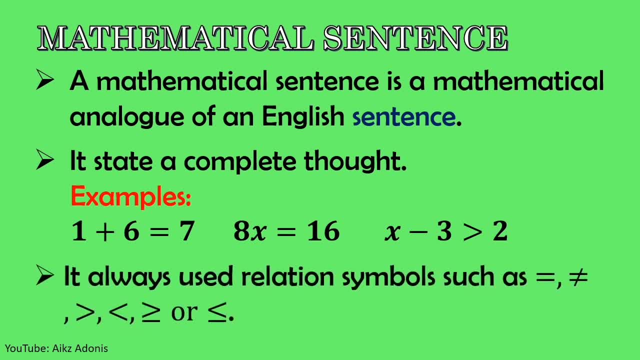 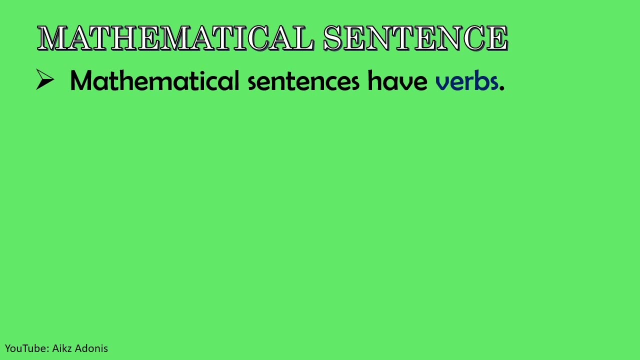 Mathematical sentences always use relation symbols such as equals, not equal to, greater than, less than, greater than, or equal to, or less than or equal to. Also, mathematical sentences have verbs In: 1 plus 6 equals 7, the verb is equal. 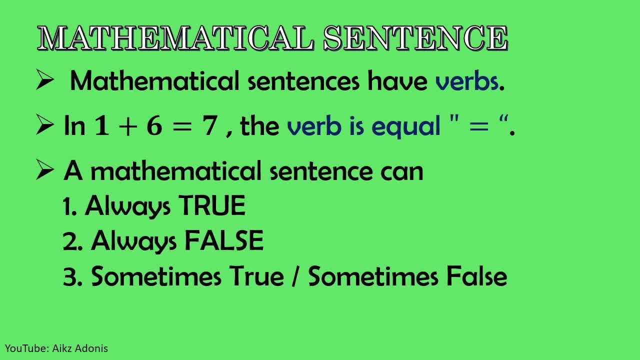 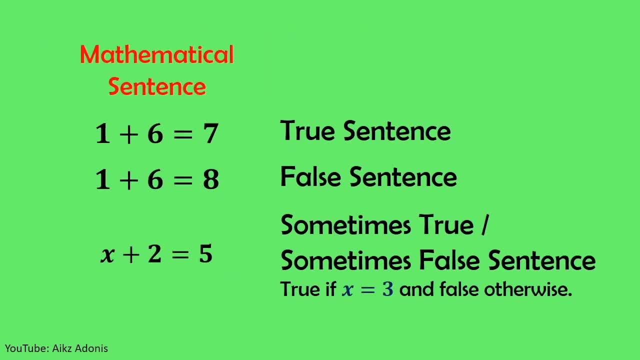 And mathematical sentence can always be true, always false, or sometimes true or sometimes false. In the mathematical sentence, 1 plus 6 equals 7,. this sentence is a true sentence, while 1 plus 6 equals 8 is a false sentence. 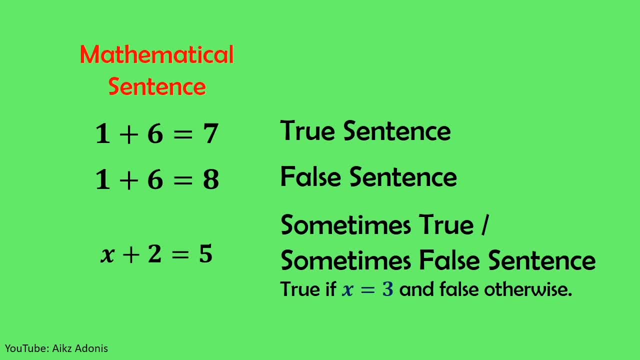 And x minus 3 is equal to 16,, 8x is equal to 16, and x minus 3 is greater than 2 are mathematical sentences. In the mathematical sentence, x plus 2 equals 5 is a sometimes true or sometimes false sentence. 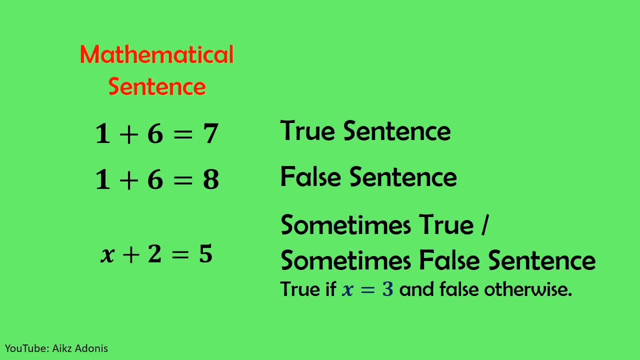 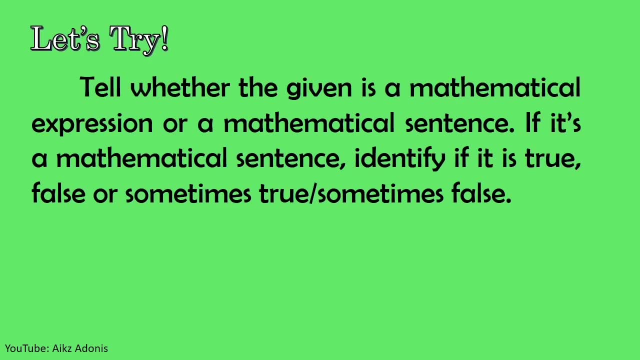 It can only be true if x is equal to 3, and false otherwise. Now let's see if you really understand the difference between a mathematical expression and sentence. I will pose something and you will tell me if it is a mathematical expression or a mathematical sentence. 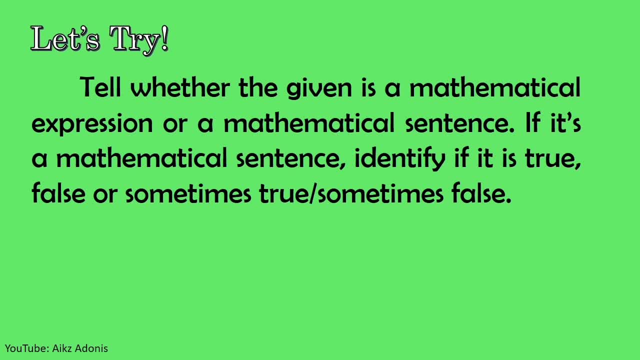 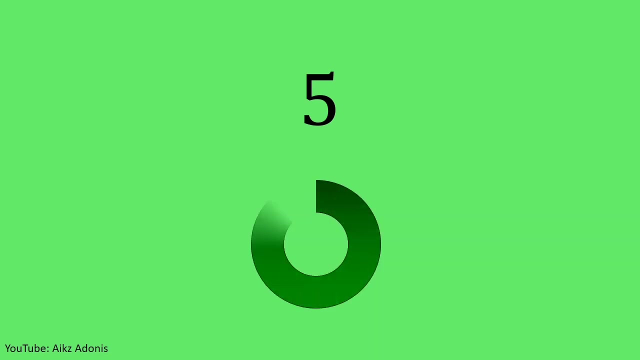 If it is a mathematical sentence, you will tell whether it is a true sentence or a false sentence, or a sometimes true or a sometimes false sentence. Are you now ready? Let's go. Let's go. So what's your score? You can also comment your score below. 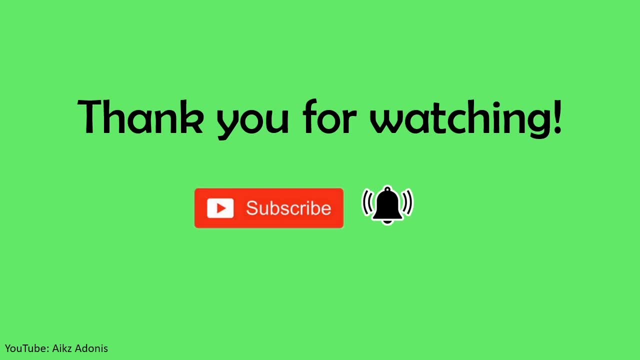 And if you get a perfect score, wow, you are so amazing. It only proves that you really learned from this video. And if you like this video, please don't forget to click the subscribe button and click the notification bell for more interesting videos. Thank you for watching.